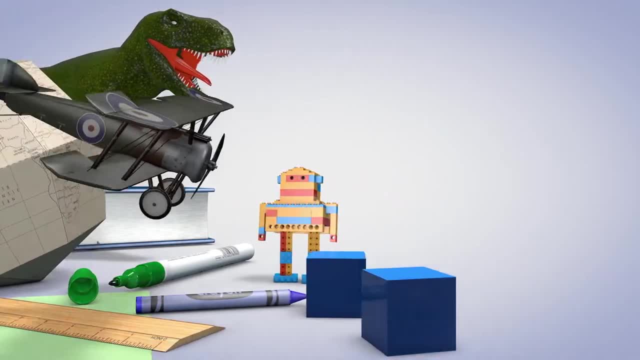 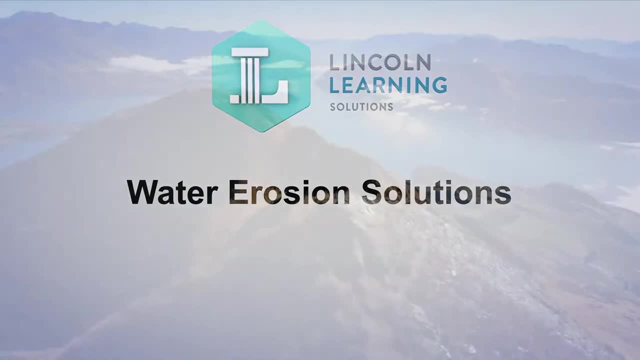 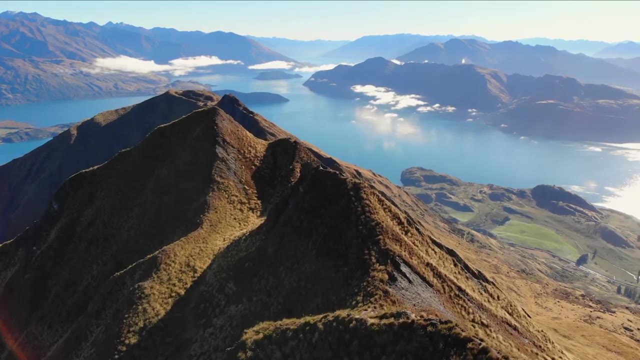 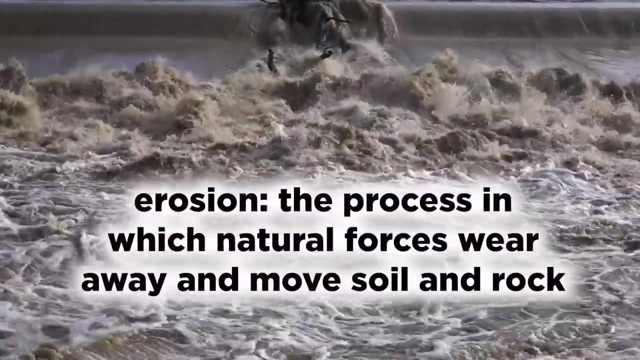 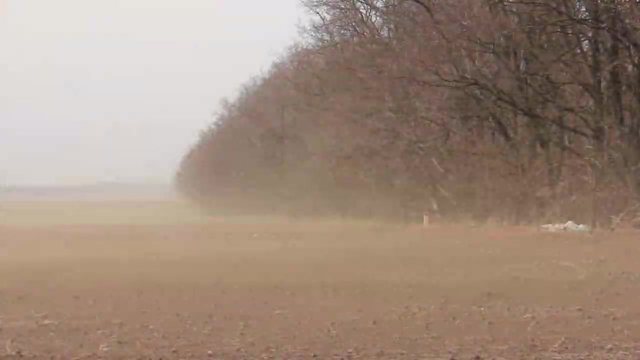 Earth is made of rock, soil and other solid materials, But did you know that Earth's surface is constantly being broken up and moved around? Erosion is the process in which natural forces wear away and move soil and rock. Two very strong forces that cause erosion are wind. 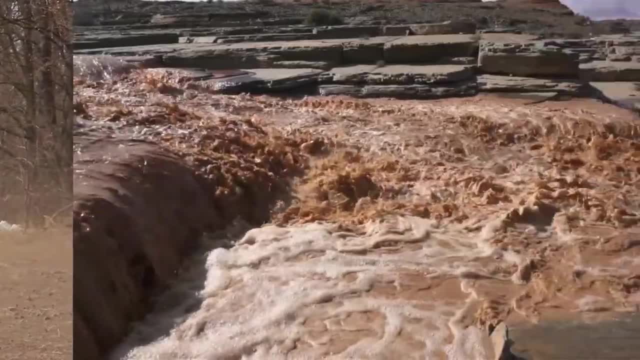 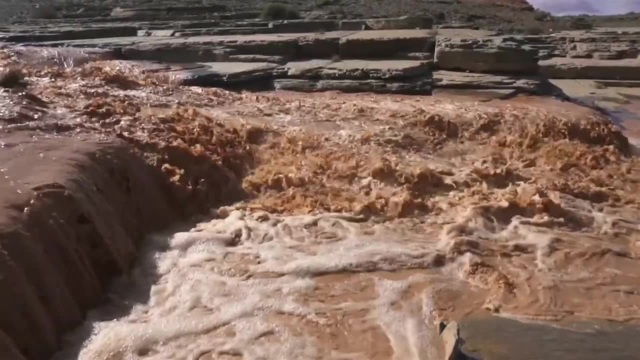 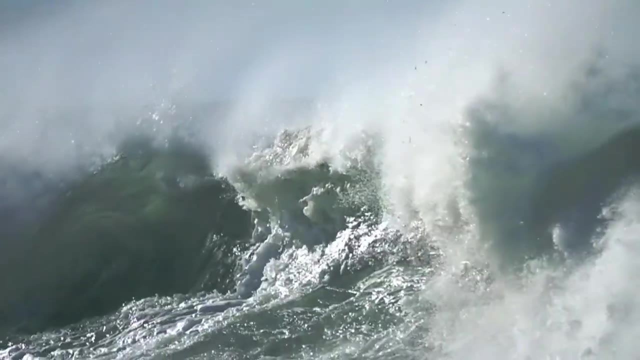 and water. Water erosion happens when running water washes away the solid materials that make up Earth's surface. This running water can be rainwater, streams, rivers or even ocean waves. Soil erosion can cause problems. For example, crops have trouble growing when topsoil is. 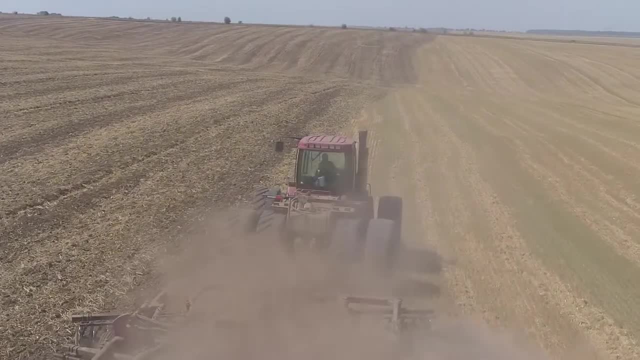 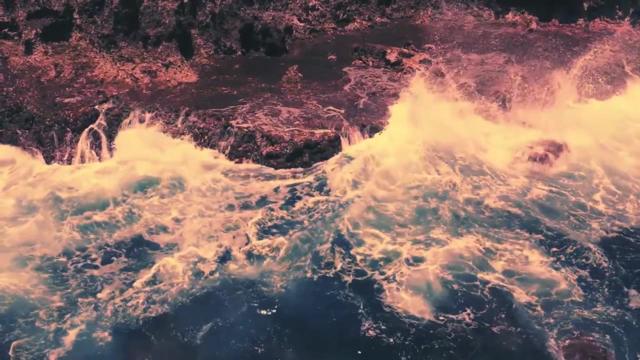 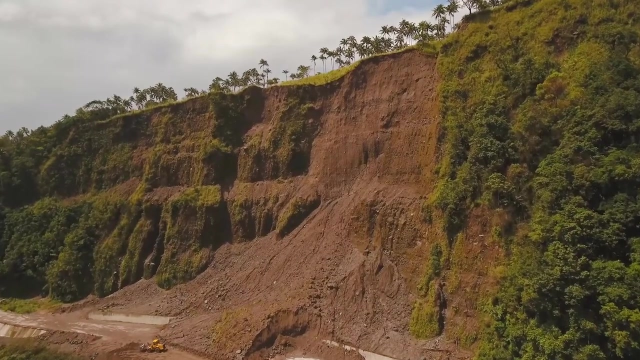 washed away from farming areas. This is a common problem for farmers. Soil erosion can also cause more pollution in waterways. In addition, soil erosion can lead to landslides, flooding and other damaging events. These events are often dangerous and costly. 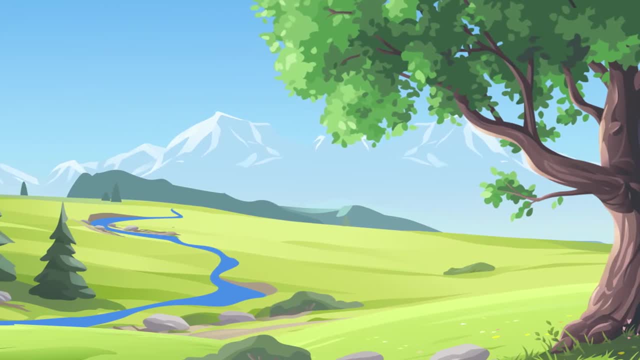 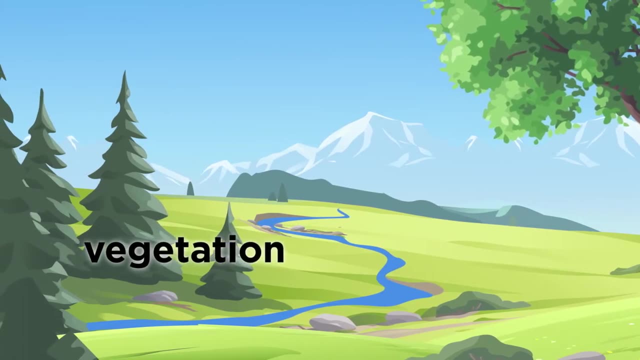 There are several ways to prevent water erosion. One of the easiest solutions is to add new vegetation or plants. Plants help stop water erosion in a few ways. First, their roots grow down into the soil and hold it in place. The parts of the plants that are above ground also help by slowing. 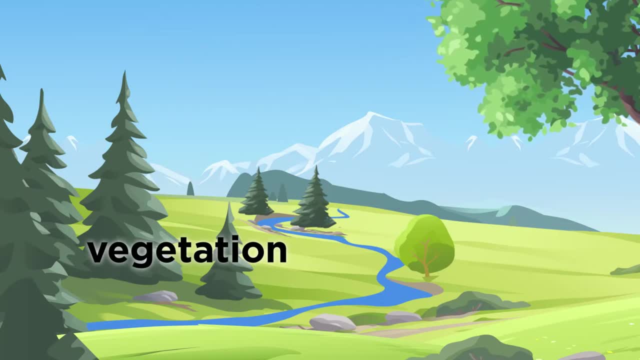 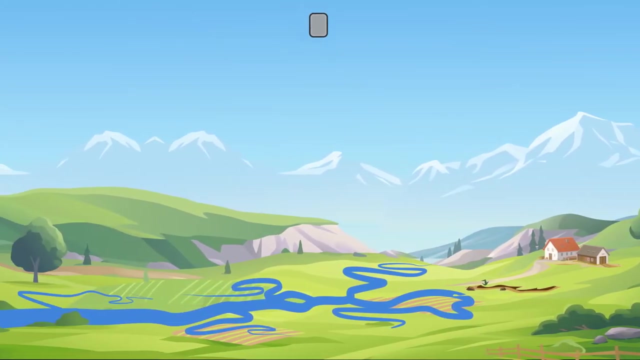 down the flow of water. This keeps the water from washing away. soil Plants also absorb water. The less water that runs off an area, the less soil erodes. Another solution to stop soil erosion is to build a structure. A dam is one type of structure. 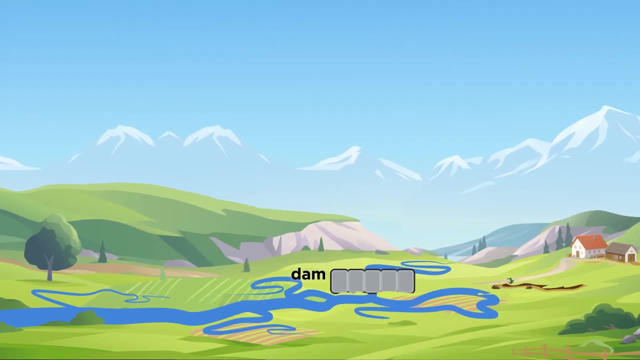 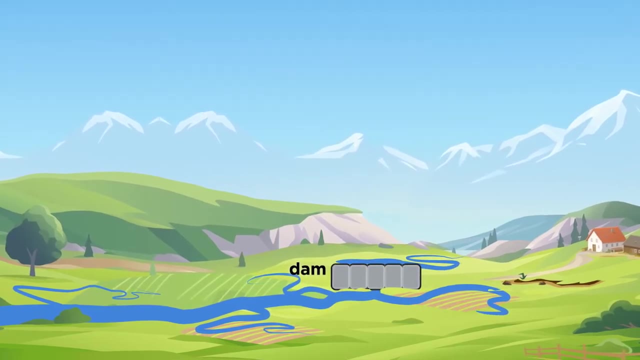 It is a barrier that stops or slows the flow of water. Dams can be small or very large in size. They are built across the flow of water, which keeps the water on one side. Dams help prevent flooding in areas where water runs out.